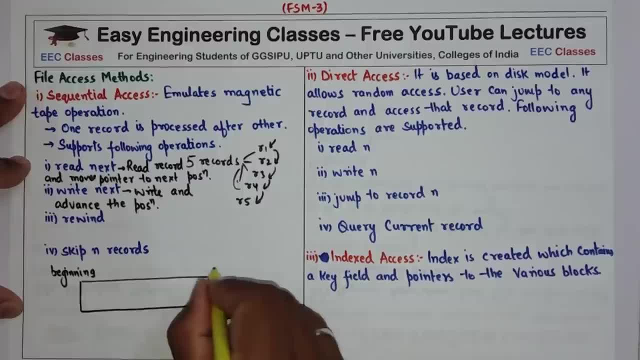 and this is the end of the file and, for example, currently we are at this position. so this is the current position. so if a user wants to come back, then the user needs to, then the user needs to issue the rewind operation command to come back to the beginning position and to move in the 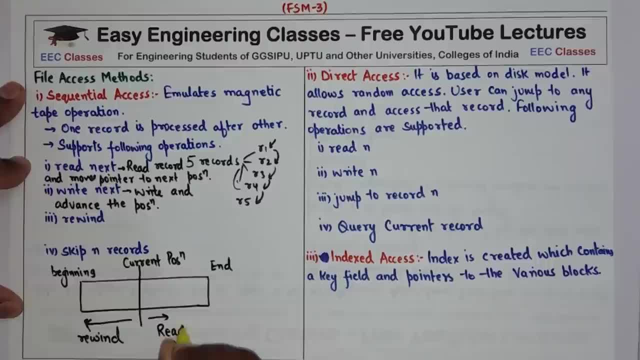 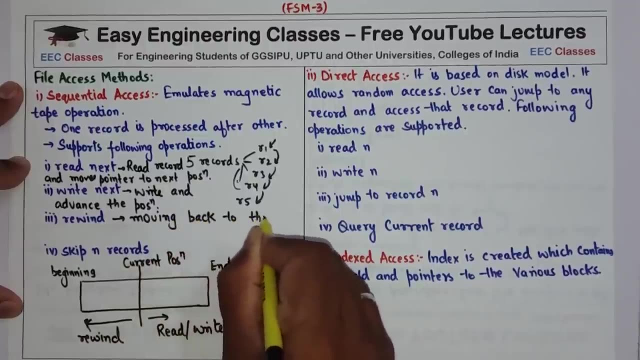 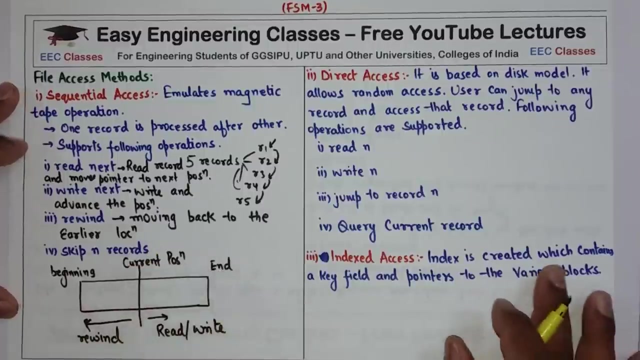 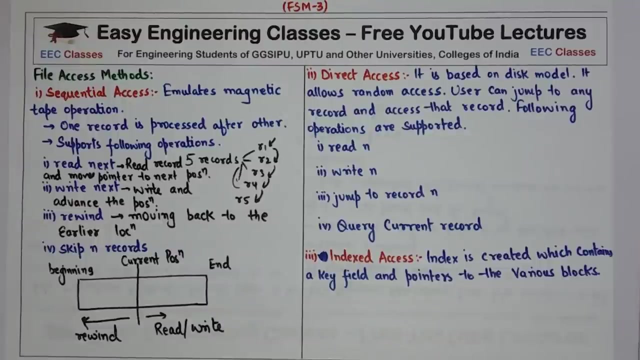 forward direction. user needs to use either read or write operation. so this is rewind. it means moving back to the earlier location. it is moving back to the earlier location. then we have skip and records. it may or may not be supported by the operating system. it means we can skip n number of records. so 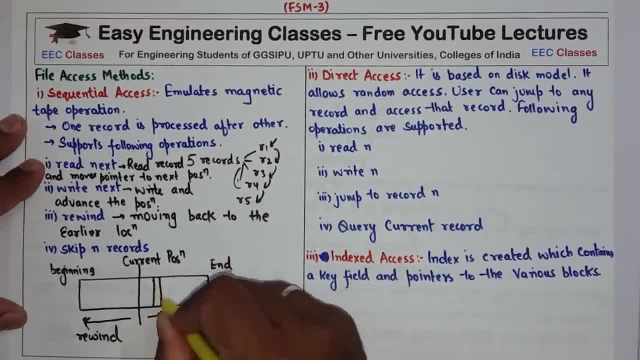 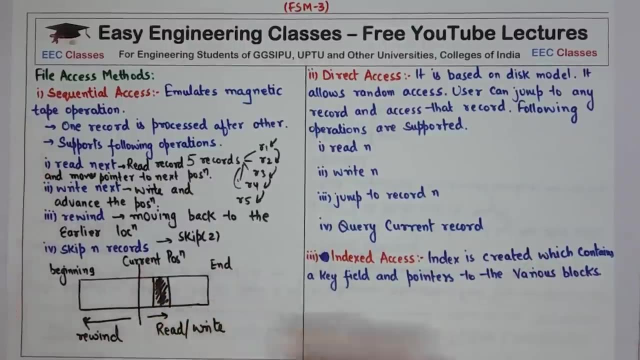 for example, if there are two records in between, like this, and if I am saying skip to from current location, and if this operation is supported, then these two locations will be skipped. so this, this skip, depends on the type of operating system you are using. this is your sequential access. then we have direct access. it is based on the disk. 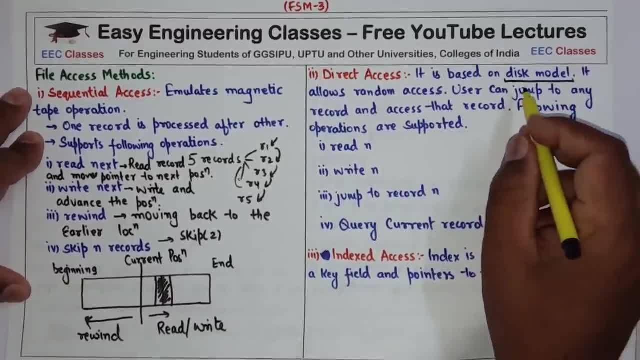 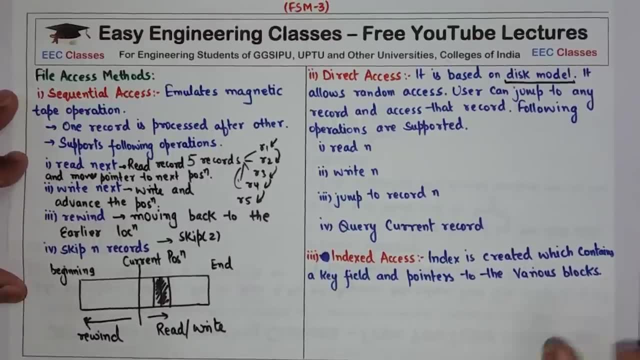 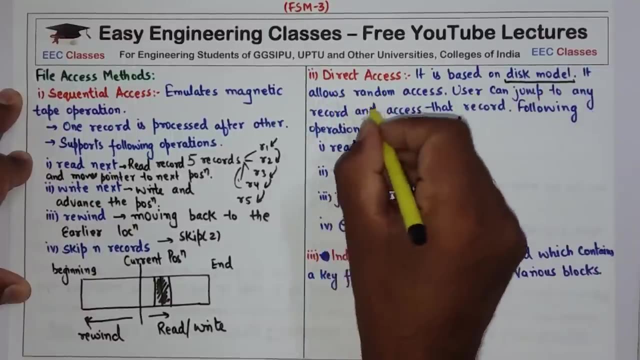 model as we have already seen that in disk we use the concept of blocks and blocks can be accessed randomly or we can directly access any block at any time. so this direct access is based on disk model. it allows random access. user can jump to any record and access that record now. following operations are: 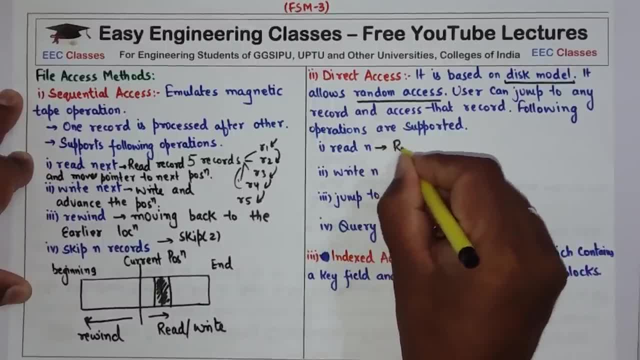 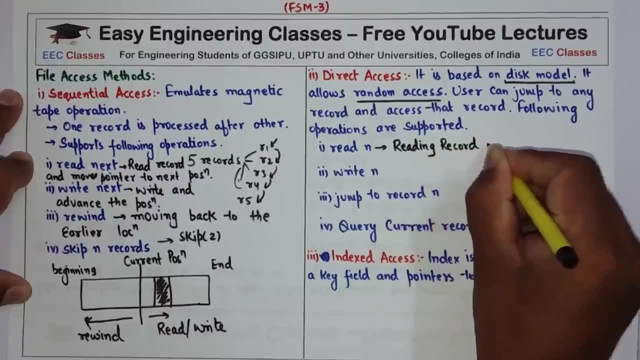 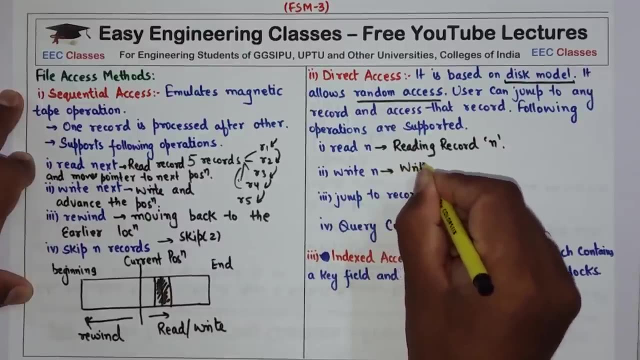 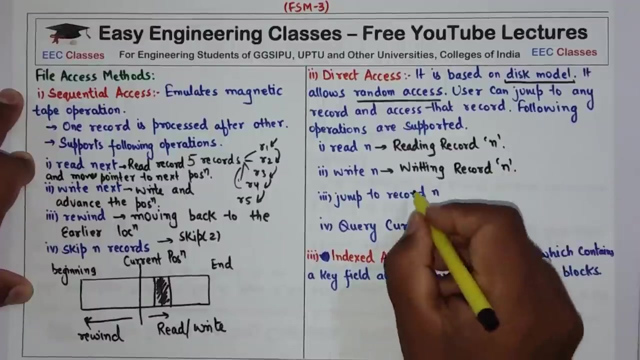 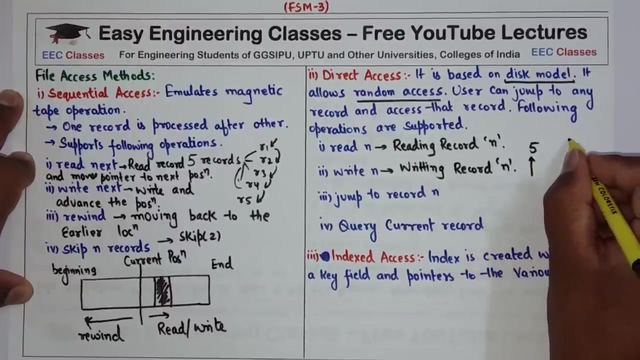 supported. read n means reading reading record number n. reading record number n. then write n means writing record number n. jump to record and means: if suppose currently we are at record number five and we want to access record number 10, then i can use jump to 10 from 5. it means it will skip. 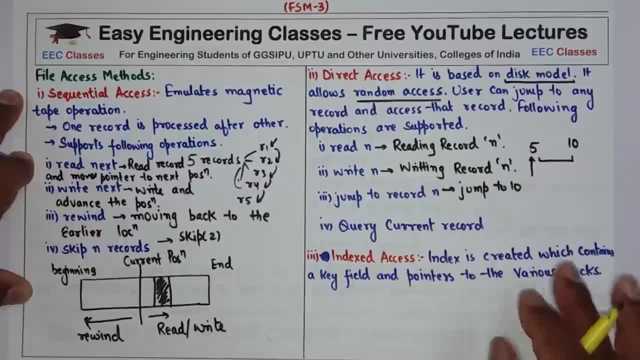 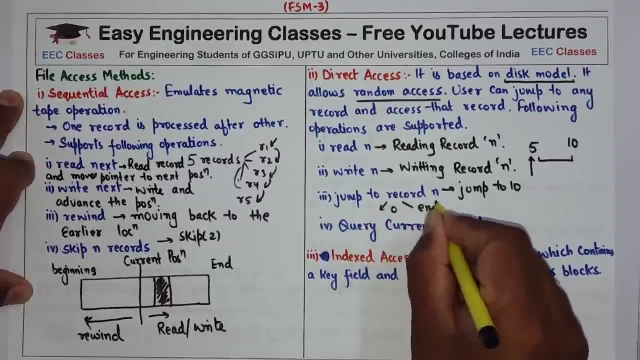 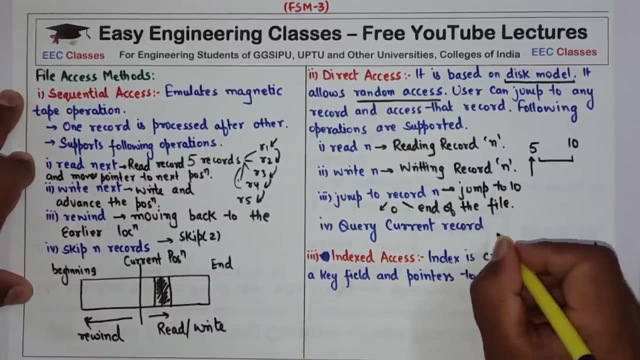 all the records in between 5 to 10 and directly jump to record number 10, and it can also be 0 or end of the file. then we have query current record. it is used to return back to this record later. used to return back to this record later. 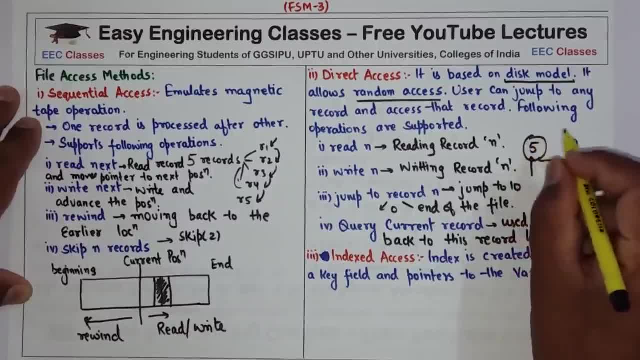 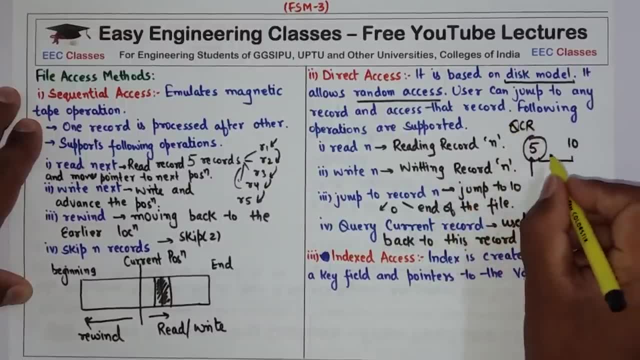 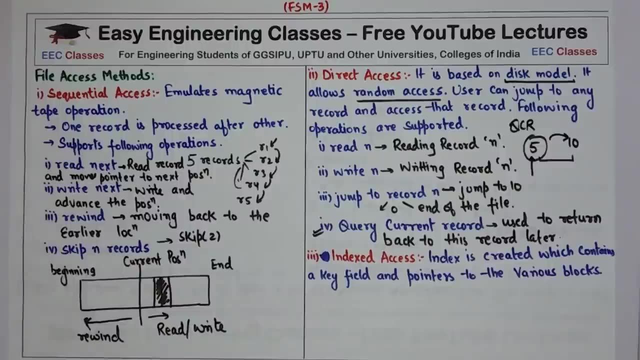 now, for example, user is at record number 5 and at this record, user issue query current record. so i am saying qcr and then it moves to record number 10. then the user can use this particular operation to come back to this particular record, number 5.. so this is your direct access method, which is based on the 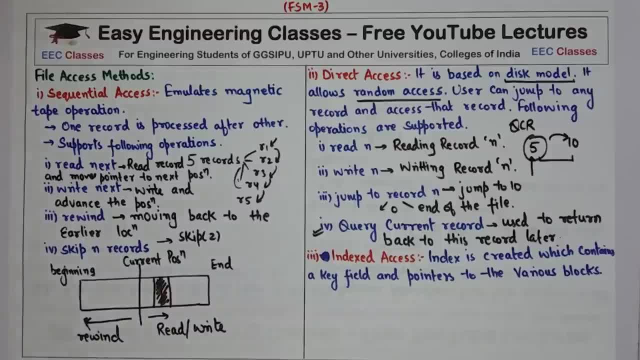 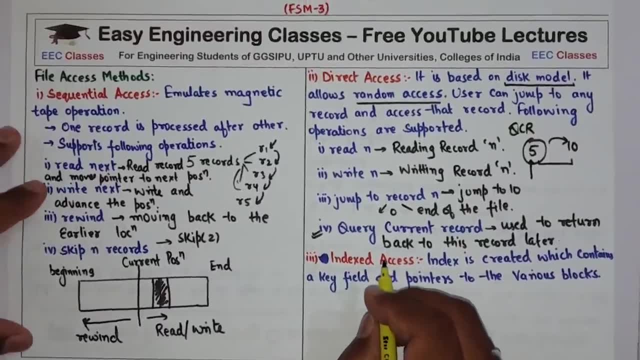 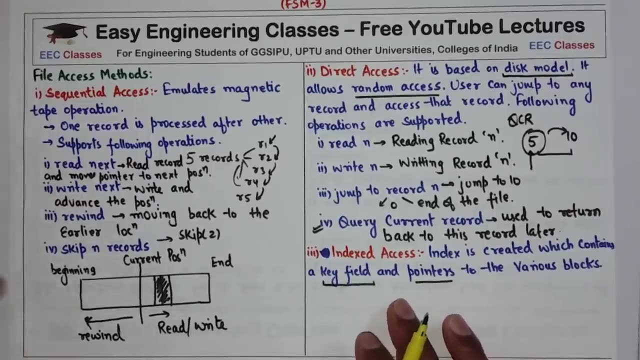 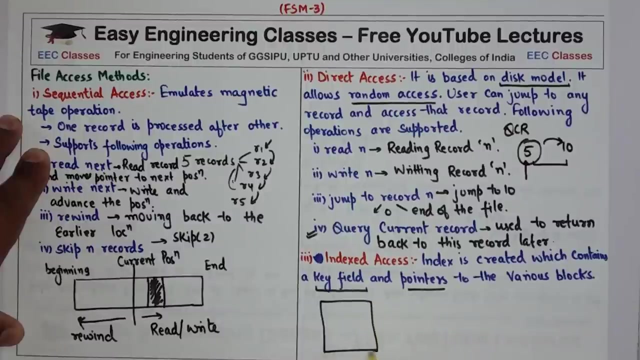 disk model. then the last is index access method. in this the index is created which contains a key field and the pointers to the various blocks. so it contains key fields and pointers to the various blocks. for example, there is an index like this: first is your key field and then we have the pointer to the disk location. 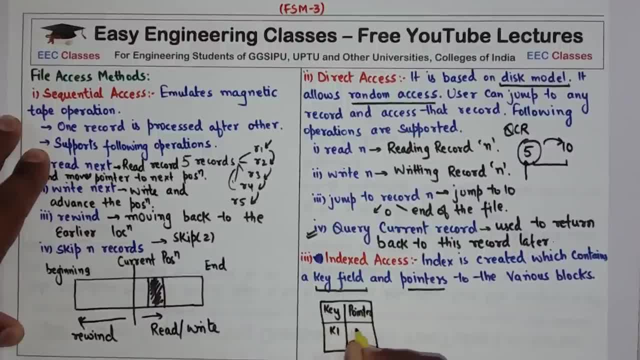 suppose key fields are like this: k1 and some location, k2 and some location, and these pointers are actually mapped to the memory at which the file is stored. so the entry for this file is at this particular location with all the entries like name, row number etc. 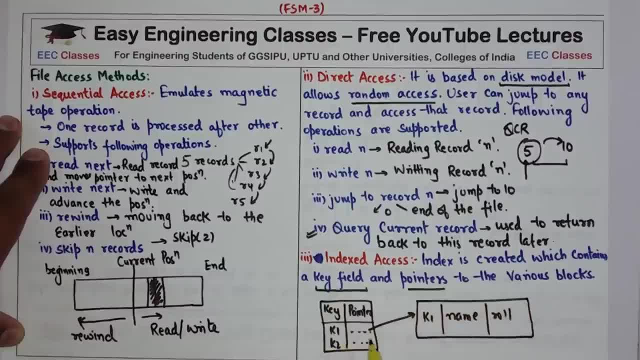 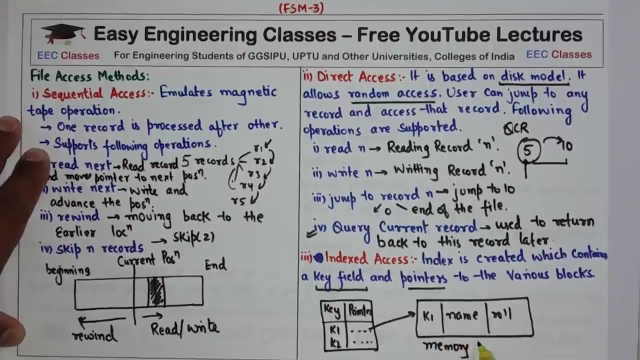 so this is based on key field and pointer. so if you have to access a file, then you have to access the index file, search for the key field and then, from the pointer, you have to access the memory location at which the file is stored. so that is how you can use index access method of. 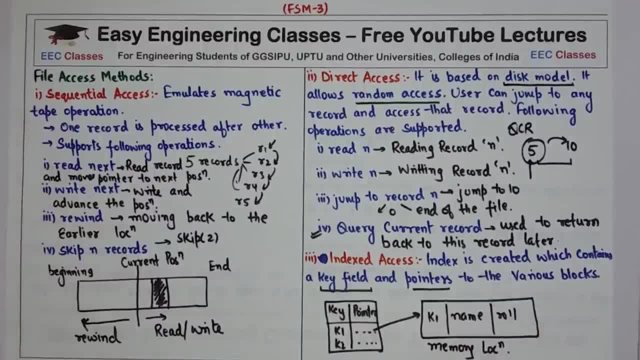 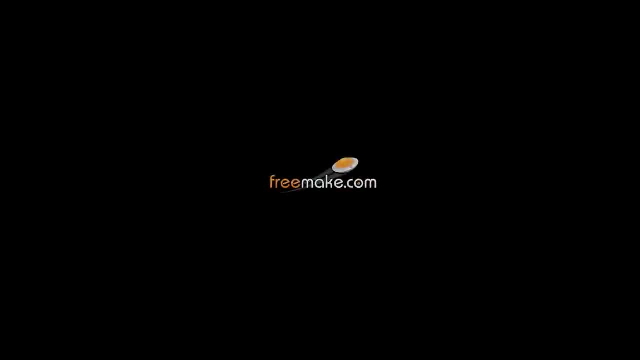 file system management. thank you for watching the video. please subscribe to my youtube channel for more such tutorials. thank you.